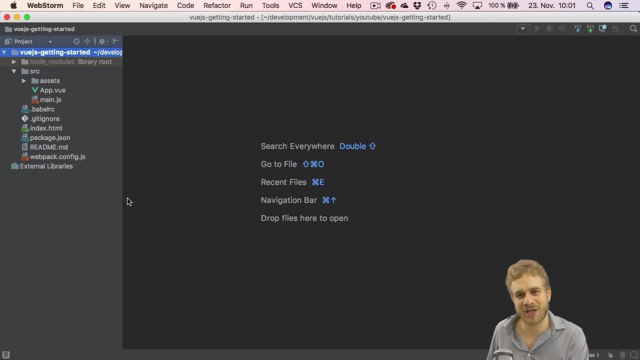 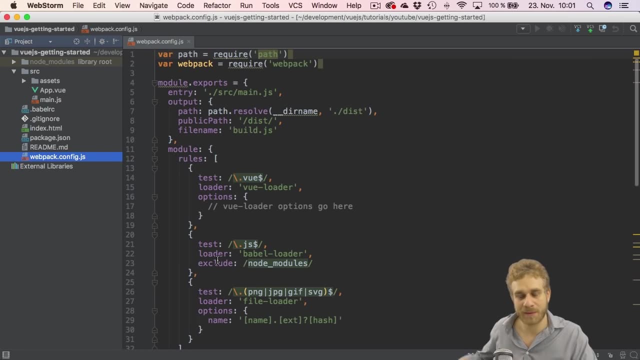 You also saw that in the source folder. we got this strange vue file here and you learned that this is basically a file handled by the Vue loader, by Webpack, here in the end, and everything is then bundled together in one file in the end. 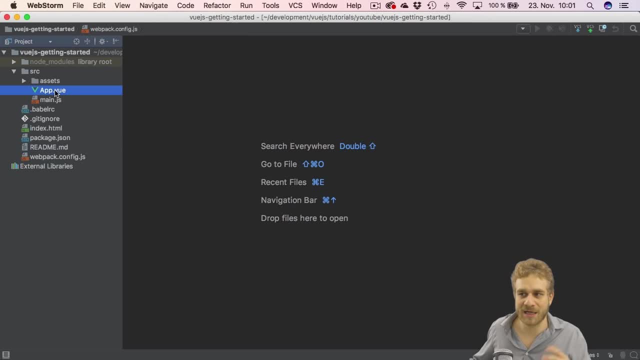 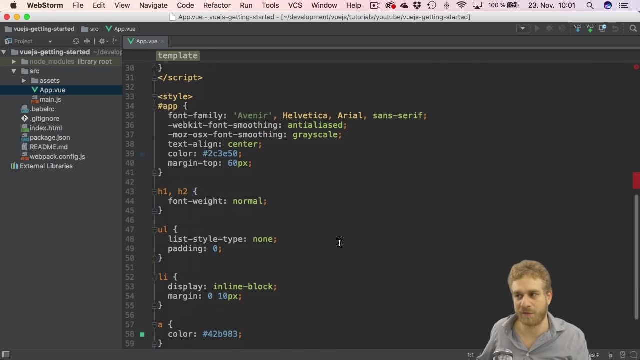 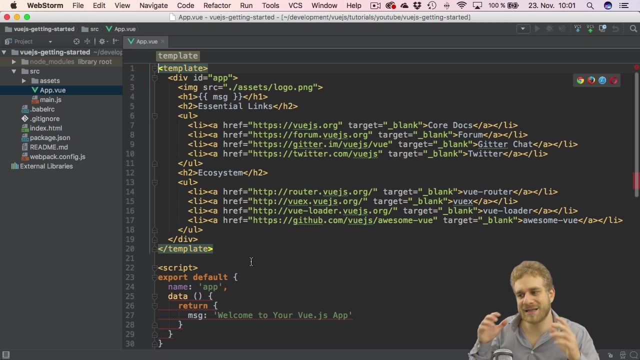 It's a nice tool to be able to split up our code, though In this vue file we got three different sections: the template, the script section and the styles of generally applied to the whole app, but can also be scoped To this file here, also of this template, and that is a convenient way to be able to split up our code over multiple files. 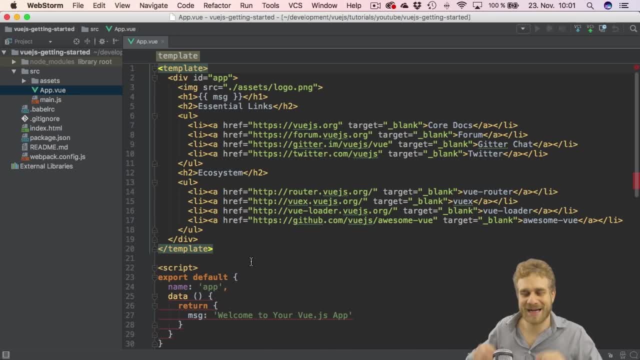 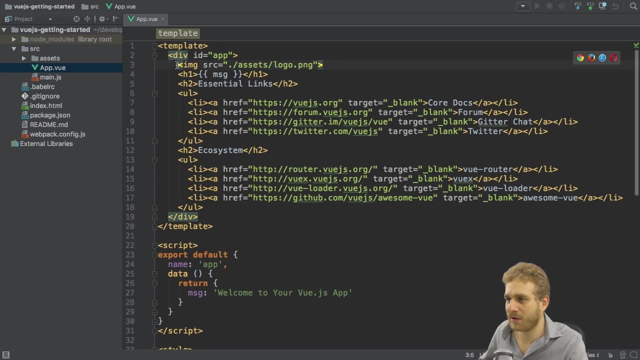 Now, in this video, I'm going to have a closer look at how we can use these files, how we can split up our application over multiple files using components. Now let's take a closer look. We already have the appvue file, and I'm first going to get rid of all the content in there. 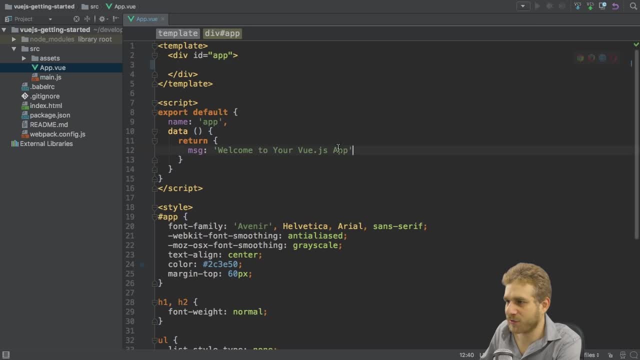 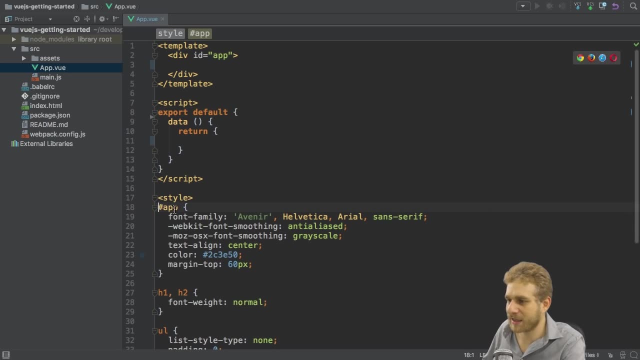 This standard content. I'm also getting rid of the content in my data field here. I don't need the name of this component, kind of I don't need to name it, and I can also strip out all the styling. in the assets folder where we have this logo, I can also delete that. 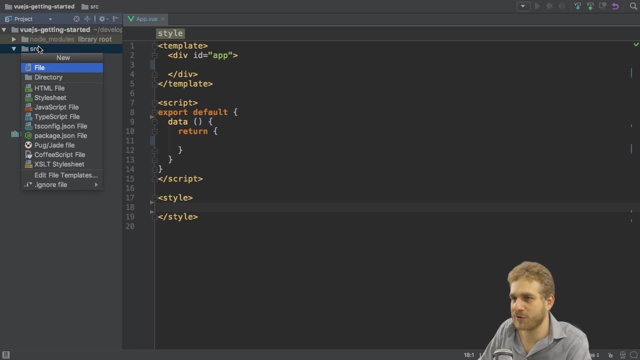 Now, if we have a look, this is much leaner. and next I want to create a new component. I will do this by creating a new file and I will give this file the name of well, of the component, the name my component shall have. 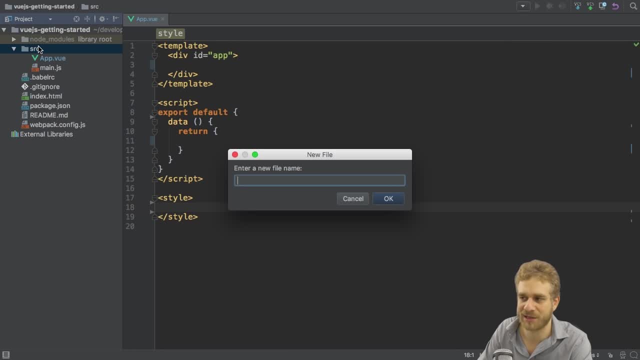 That's just a naming click And then I'll add in a new version which is kind of used in the Vue JS world. So let's say, here we wanted to create a symbol, a simple message component, So messagevue file, And in this file, well, we need a template. 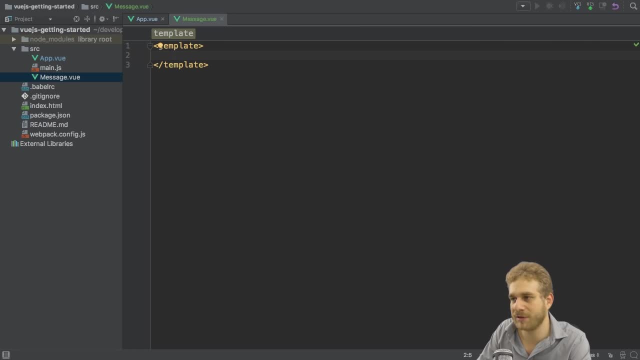 Template is something you will always need. In the template, we must only have one root element, So let's name it or let's make it of type div, And then there, I want to simply say this is a great message, whatever you like. 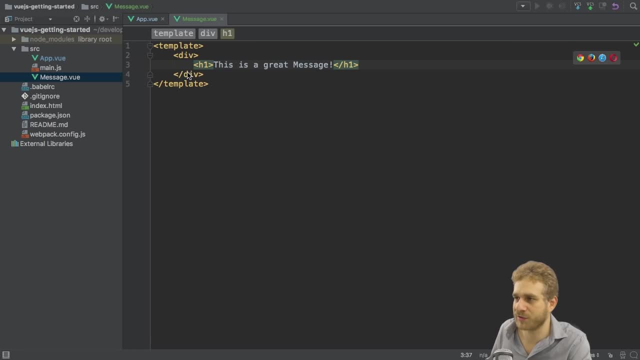 so in h1 tag here we could of course, until now also use this h1 tag as the main element here. we don't need to div as of now, since we only have one nested element now. this is this component, and i already had a video on components there. we created it with this viewcomponent command. 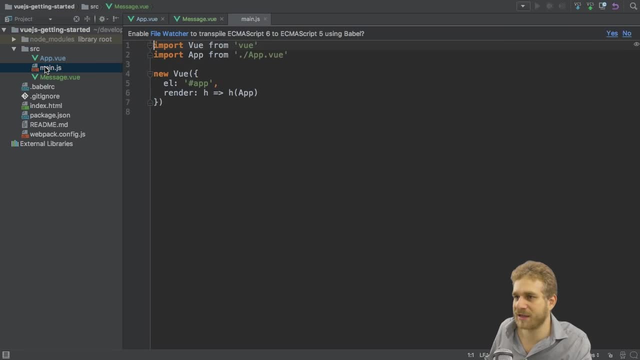 and we can still do this, however, not in this file, instead here in the mainjs file. i first need to import my messageview file. let me add semi-semi-colons because that's the style i'm using here. so i'm using or i'm importing message from messageview now, interesting enough. 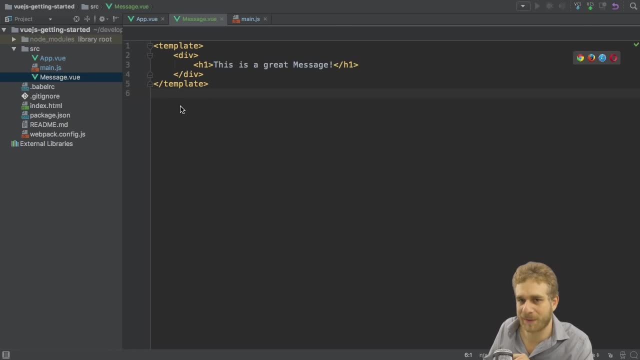 i'm not exporting anything in the messageview file. i don't have a script tag where i export anything. it will work nonetheless, because a webpack or this view loader will do this behind the scenes for us. it, as i explained, transforms this template here to javascript code anyway. 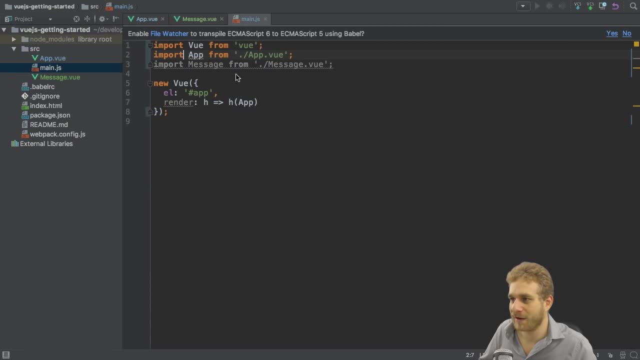 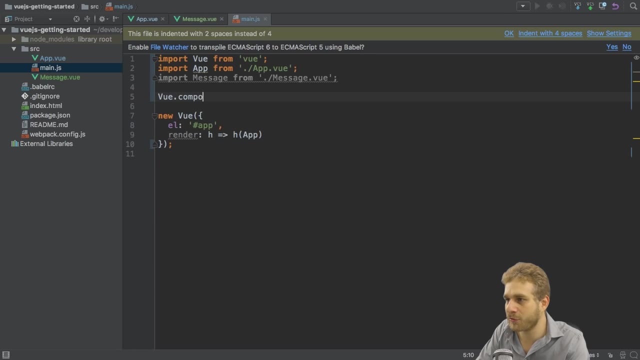 and it will export it so i can import from this messageview file. now, with the message imported, i can simply use the view component method here again to set up a new component on my view instance and give it any selector of my choice, like message, or maybe also with a unique prefix: app message for. 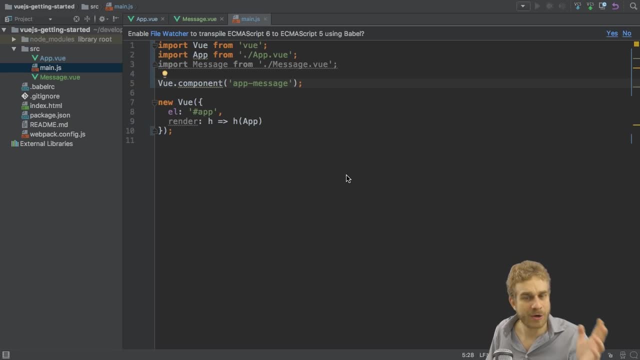 example, to make sure i'm not interfering with any third-party components i might have, or native html elements. the second element, then, simply is message, because this is my component. remember, before we had an object here where we would configure it. well, this object is now given to us. 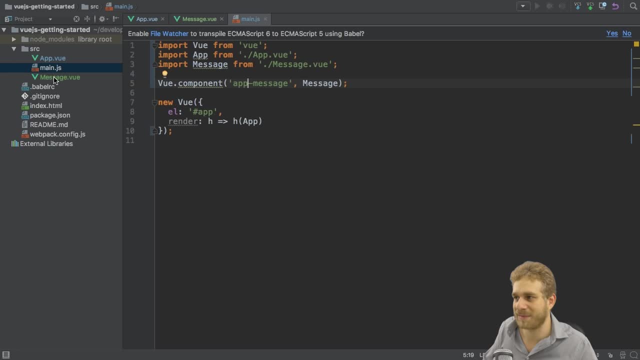 by the view loader, you could say by compiling this messageview file here now. with that i got my component registered and in the appview file i can therefore now use app message here like this, like the selector, because it is registered globally. now, if i go to the terminal and run npm, run dev to bring up my 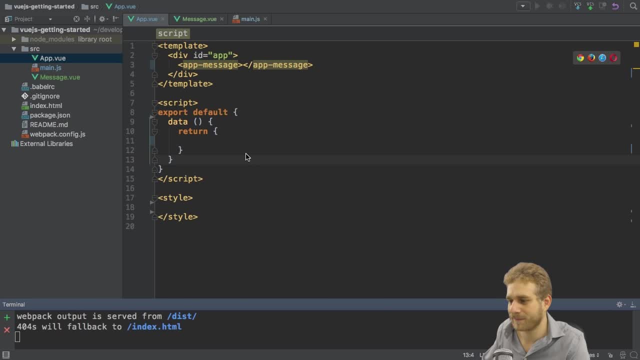 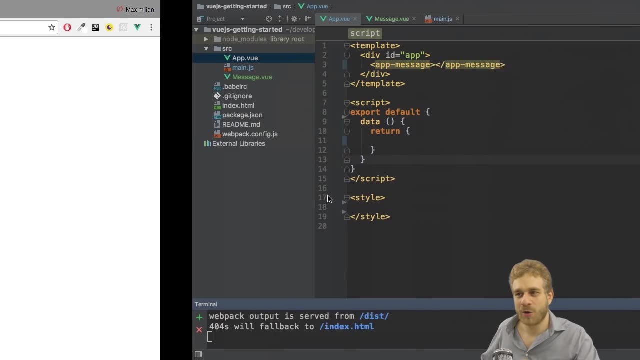 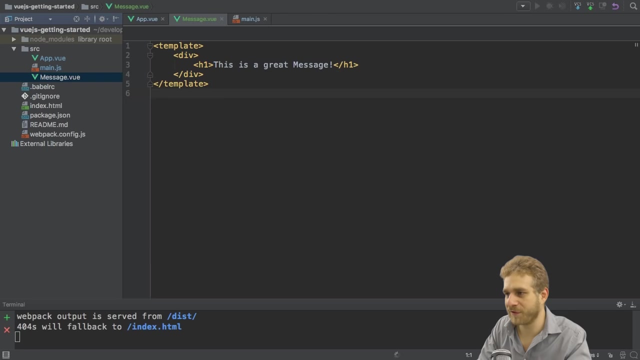 development server again. let's take a closer look. as you can see in the running browser window at localhost 8080, i got- this is a great message- using my own component, which i outsourced in the messageview file. now let's create another component. let's create the inputview file. 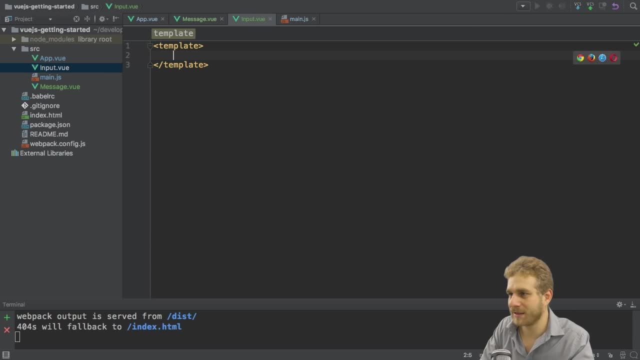 for the input component. there i'll create another template and in this template i'll again add a div. and then i want to have an input field type text here and let's also output whatever we input here below this input. well, we can use two-way binding for this with we model. 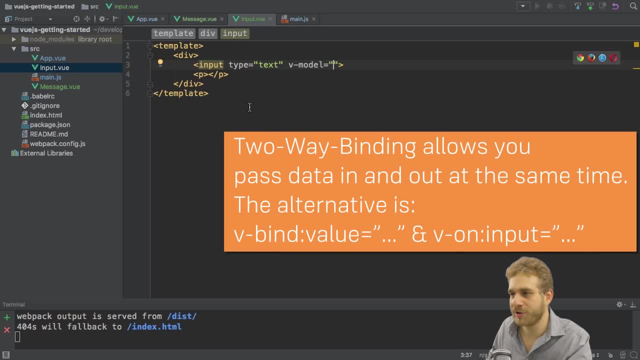 we model. we'll simply bind the content we enter here to a data property and therefore i need to add such a data property. therefore i need to add a script and here we need to export this object. and this object here is now set up like a view instance, kind of like a view instance. so i'm going 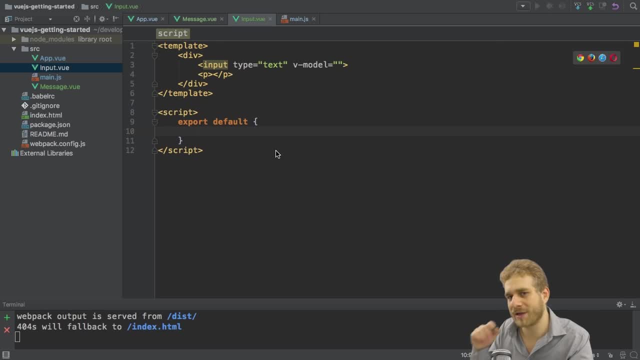 to show you how to do that. so i'm going to show you how to do that. so i'm going to show you kind of. i will show one important difference, which i already talked about, though, in the components video. here we set up data as a method, and i can use es6 syntax for that. so the alternative would be data colon function. 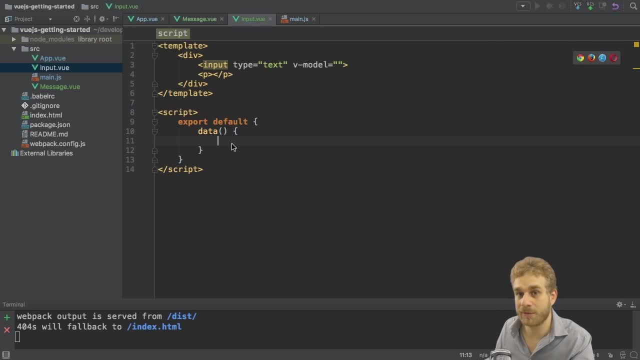 or just again, the shortcut es6 gives me which i can use here, because another nice feature of this webpack template i'm using: it will compile es6 code to es5, so can use es6 here. now, with this setup, with this data here, i need to return an object in here which i'll name. 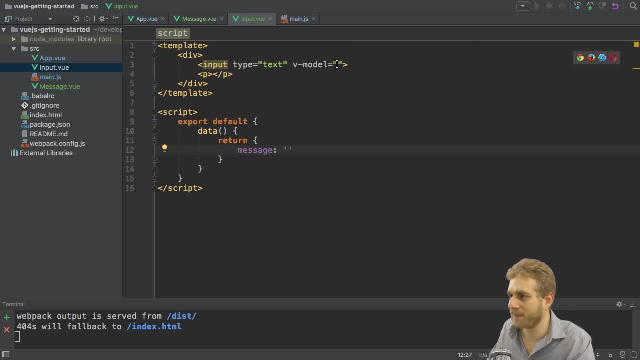 message and should be empty at the beginning. now i want to bind my input here to this message property with the model, again for two-way binding, and thereafter i can output it in the paragraph below. now i also have to register this, and to register this i could of course again add it. 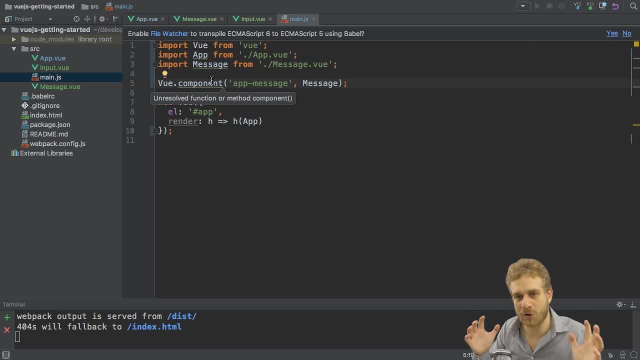 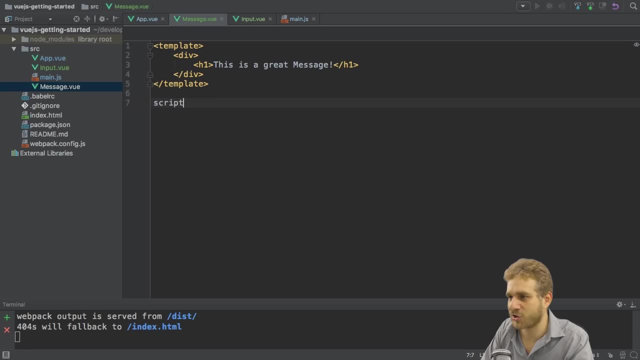 here with view component in the mainjs fault to create a global component or if i don't know, i only am going to use it here in my message. well then, i can just add a script tag here too, export an object here too and add the components property to register some local. 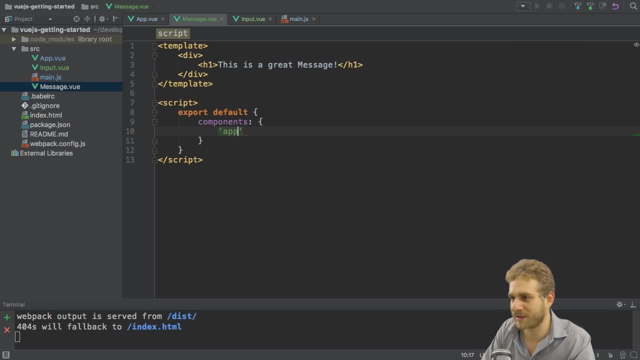 components. here the keys are the selectors, for example app input, and then the other. the value would be the component itself which i of course have to import, so import input from, and then it's going to be the component itself which i of course have to import from the inputview file. 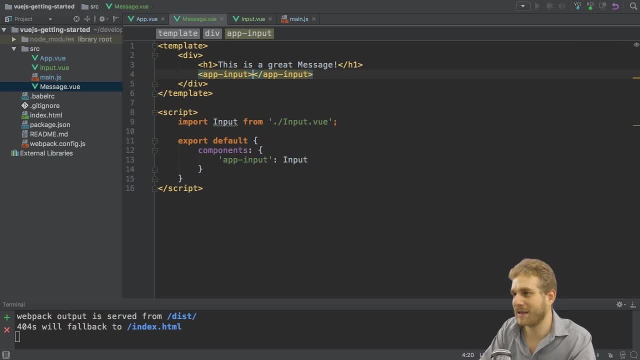 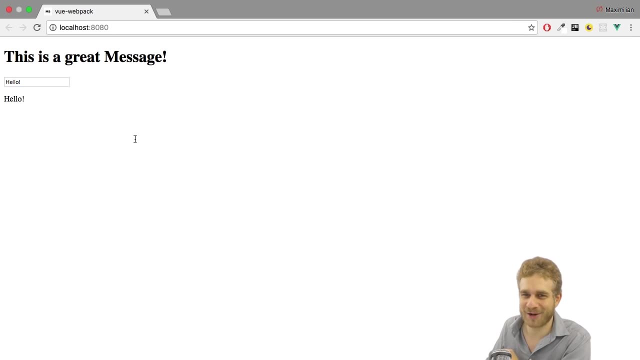 and i will then assign this as a value here, which enables me, of course, to now use app input as an element here, and if i save this and go back using the input field, and if i enter something there, you see, hello, awesome. so with that, we're using this webpack, setup these dot.